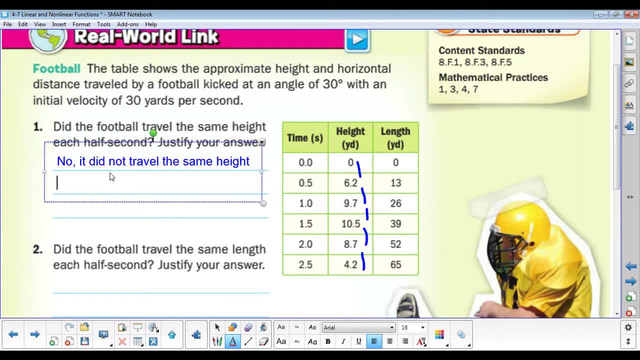 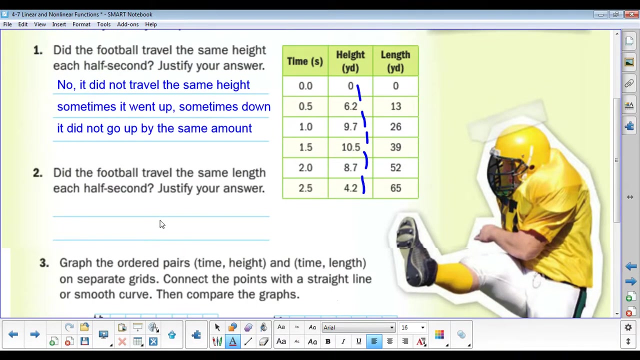 It did not travel the same height. Sometimes it went up, sometimes down. It did not go up by the same amount, So the amount is different. It went up and then it came back down, so no. Then it asks us if it traveled the same length each half second. So let's go ahead and look at that. Here it goes. 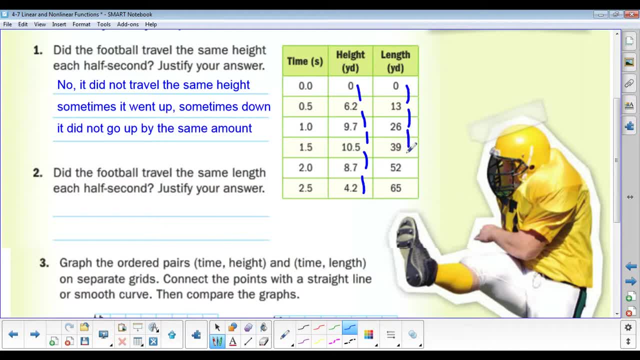 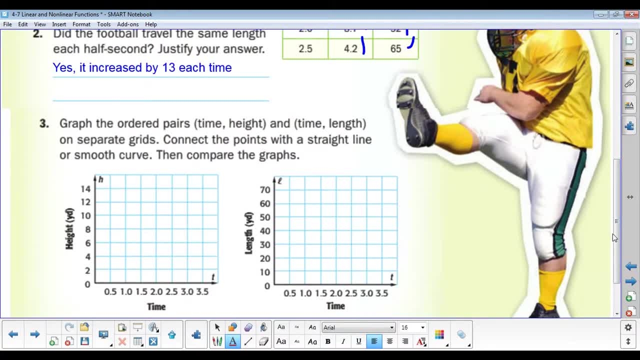 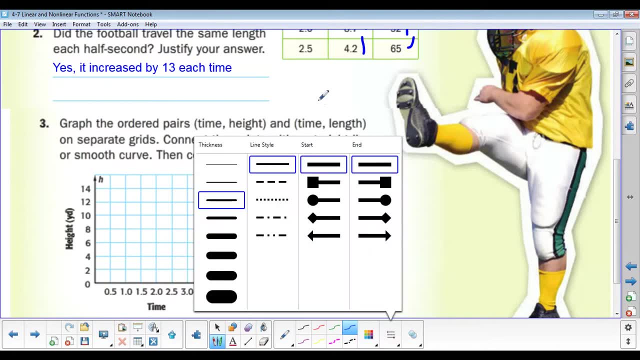 pairs, one for height and one for length, using the same time for each one. So I'm going to say yes, So I'm going to do the first one in blue And then I'm going to do the second one in red. So we 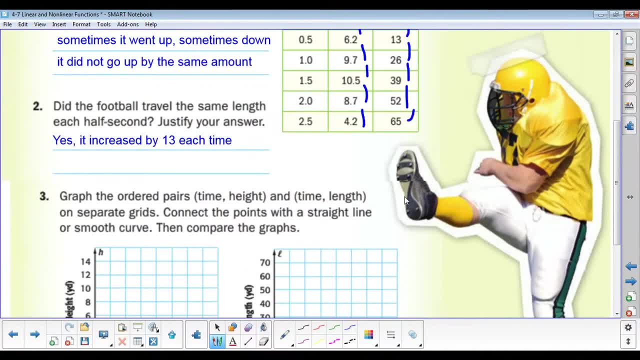 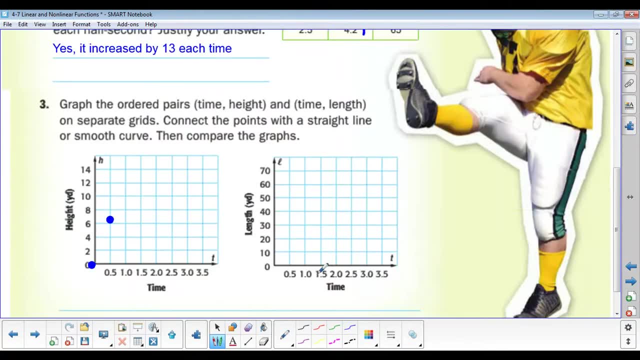 have 0, 0.. We have half and 6.2.. We have 1 and 9.7.. We have 1.5, 10.5.. We have 1.5, 10.5.. We have 1.5, 10.5.. 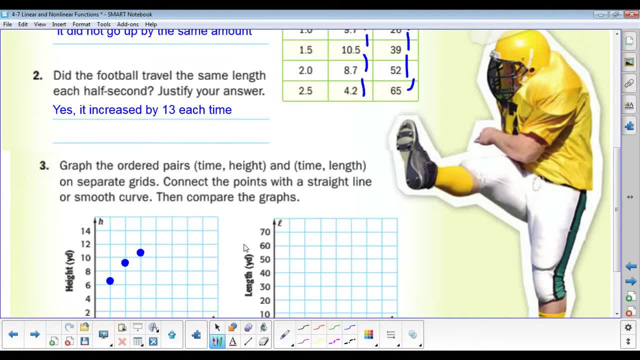 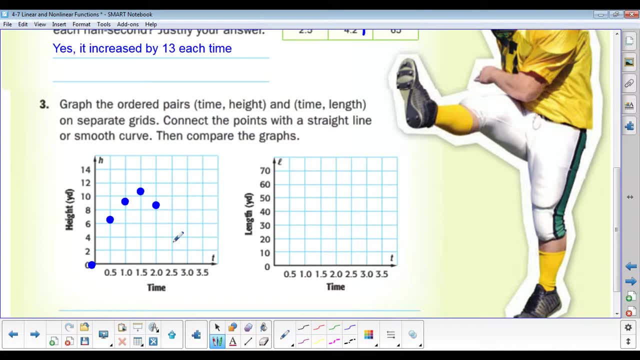 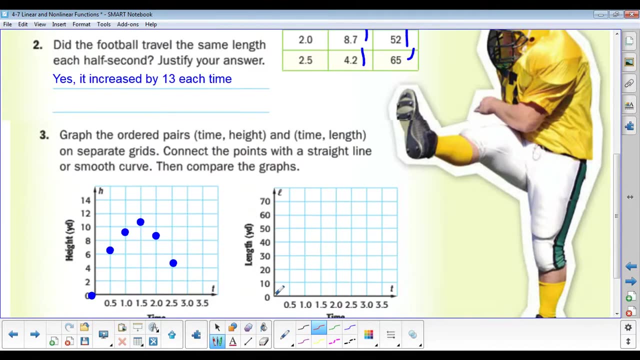 We have 2, 8.7.. And we have 2.5, 4.2. And then for the second one, we have 0, 0.. I guess I need to make this bigger again: 0, 0.. 1.5, 13. 26.. 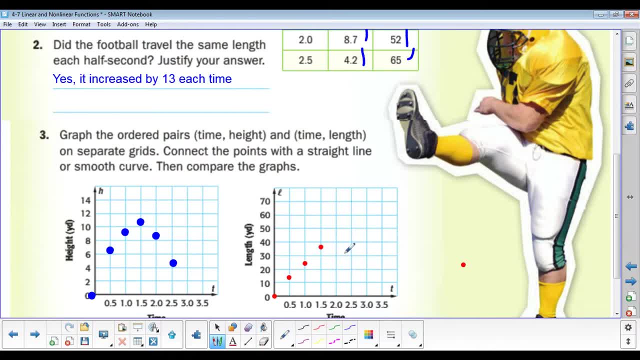 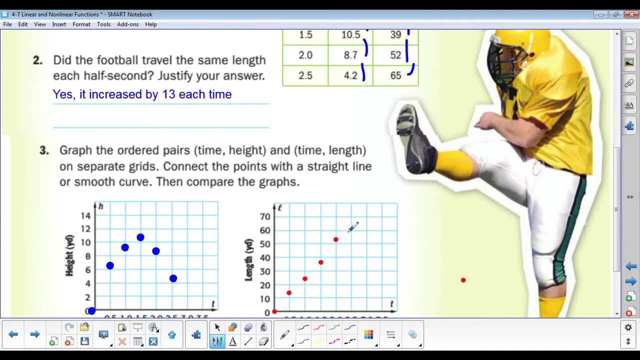 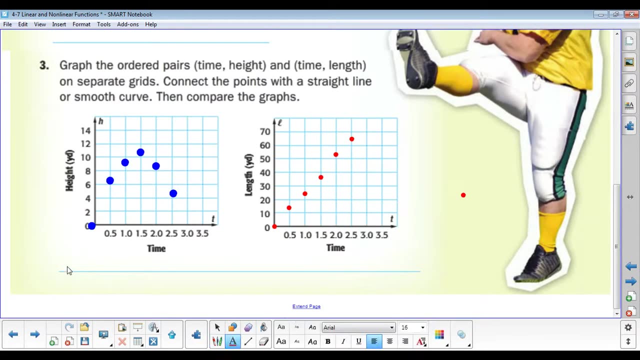 39,, 52, and 65.. So then it wants us to compare the graphs. Well, the first graph looks curved. It goes up and then down, Kind of like how you would expect something to be curved: It goes up and then down. So then it wants us to compare the graphs.